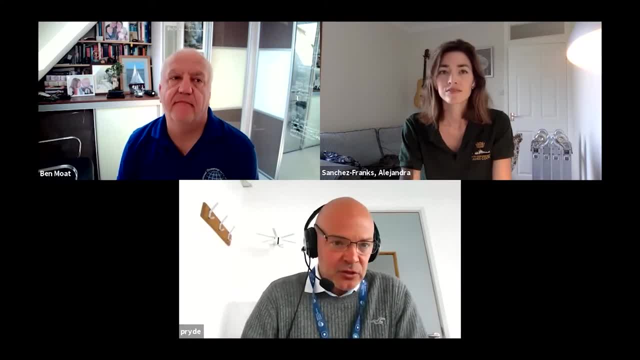 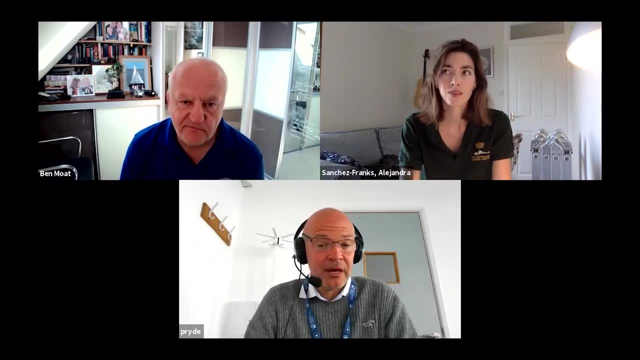 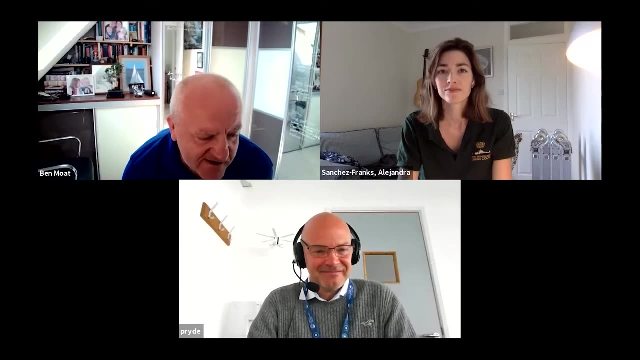 I have a few questions which we can keep the session off with, And I direct the first question to you, Ben and Ali. if you could answer the same question, that would be great. So, simply, why did you become an oceanographer? Well, okay, if I go first. So my well, my. 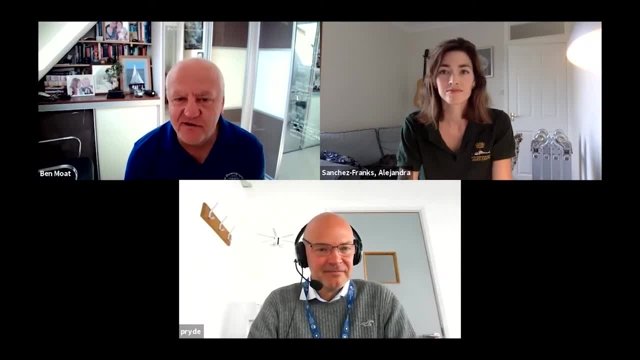 grandfather, my cousins, uncles- they were all merchant seamen And my father was a fisherman as well. So I think I was destined to have some involvement with the sea And I was very interested in the dynamics. So I went to do a degree in mathematics and then came 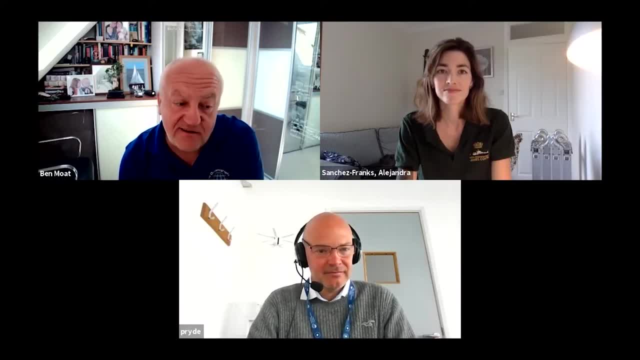 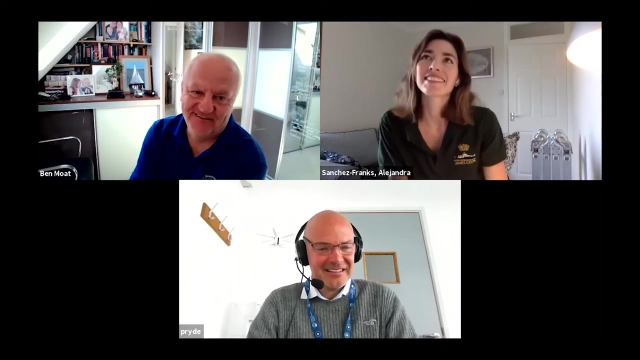 down to the Oceanography Centre here Back in 95, it was actually the Southampton Oceanography Centre then- And work paid the fees for a part time PhD, So I went on from there And then, yeah, did my PhD and I've been here ever since. Over to Ali. Thanks, Ben, I was slightly. 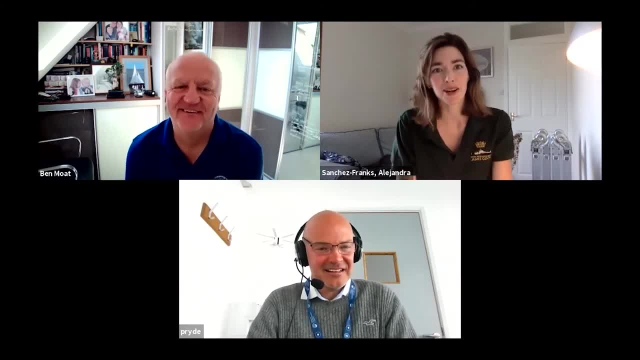 less. A lot of people have asked me about my colorful family background. that's directly related to oceanography. For me, it was mostly that I was really interested in climate change and environmental science growing up- And I mean absolutely passionate about the ocean. 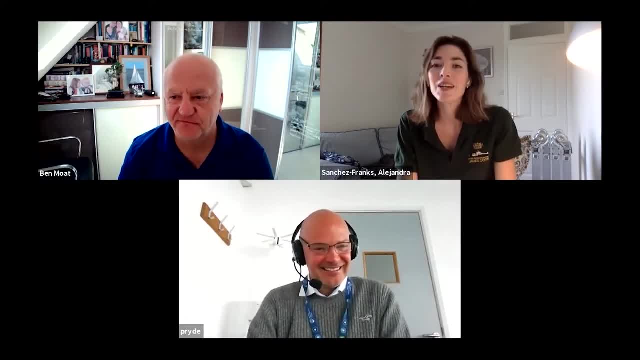 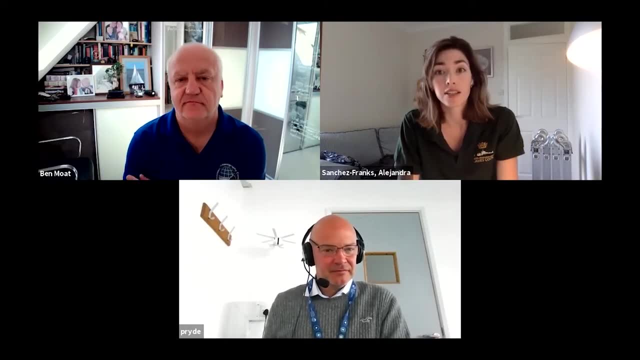 from a young age. I think most oceanographers will tell you that, But I had no idea that oceanography was a potential career path. So when I started at university, like Ben, I studied mathematics- applied mathematics in my case- And eventually I found out that 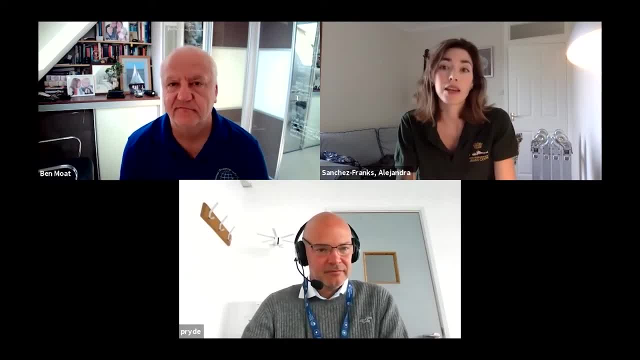 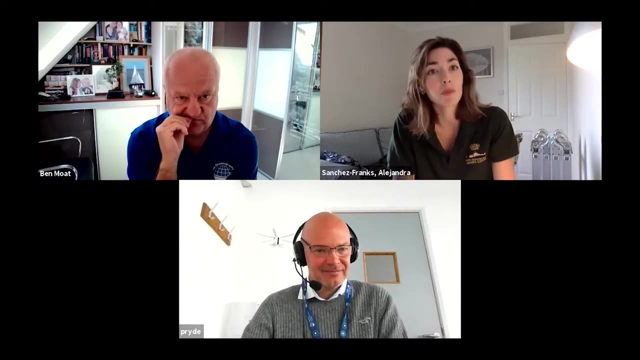 through talking to academic advisors that I could apply my background in mathematics to study and look at research questions on ocean circulation and basically I was hooked From there. I did a PhD in marine and atmospheric science and eventually found my way to a permanent position here at the National Oceanography Center. So that's a little bit both why I became an oceanographer. 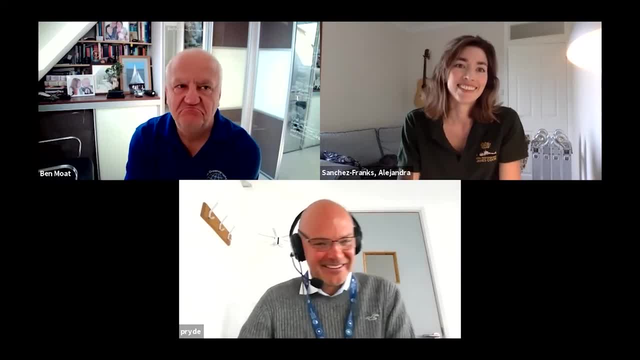 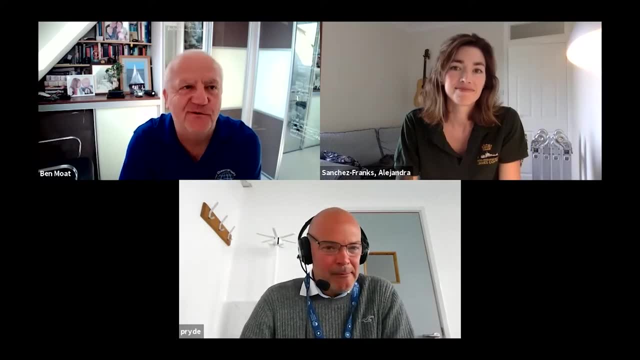 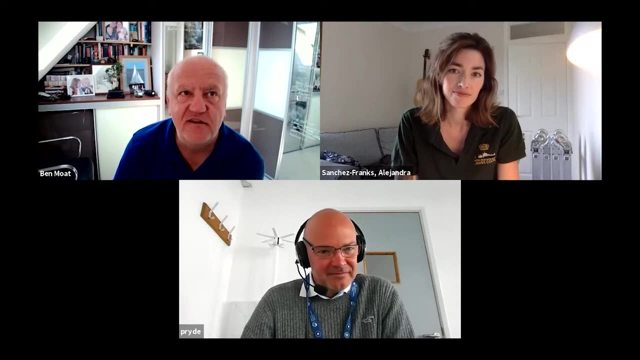 and how we became oceanographers. Great, thank you. Next question, then, is: what is your favorite ocean, and why, Ben? Oh, that's quite tricky. So I've done expeditions or been on expeditions in Indian Ocean, the Southern, the North, South Atlantic, never not the Arctic, yet actually I've. been on the edge of the Arctic Circle but I've never been up into the ice, So my favorite- I would say it's the Southern Ocean- would be my favorite, with those huge rolling seas. and I remember one time I was on the back deck of a ship heading due south, towards Antarctica, and the big swells were. 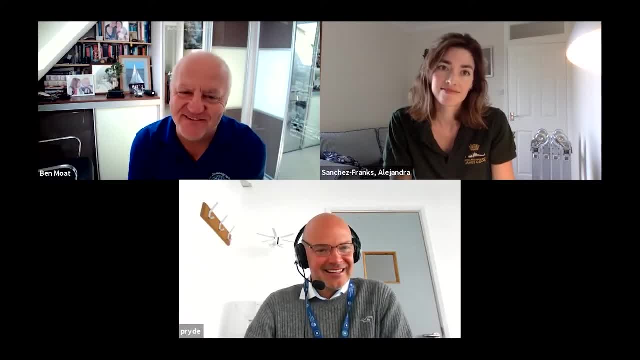 coming and I was just on the heli deck and just having a cup of tea and the sun was out and it was just marvelous. The wildlife down there is just stunning and there's so much science we can do in the Southern Ocean because it's so important for oceanography and climate. 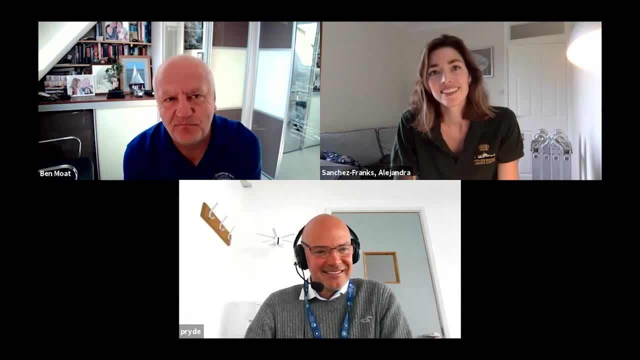 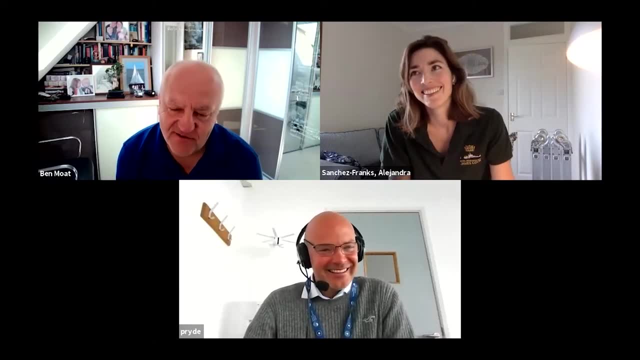 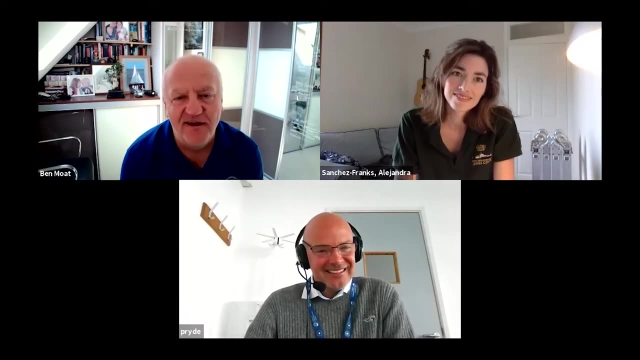 And you know generally the health of the oceans Fantastic. so you're looking to get down there as soon as possible. next opportunity: The last time I was down there was 2009 and I'm not quite sure where my next opportunity is because at the moment, like Ali you know, I'm working in the 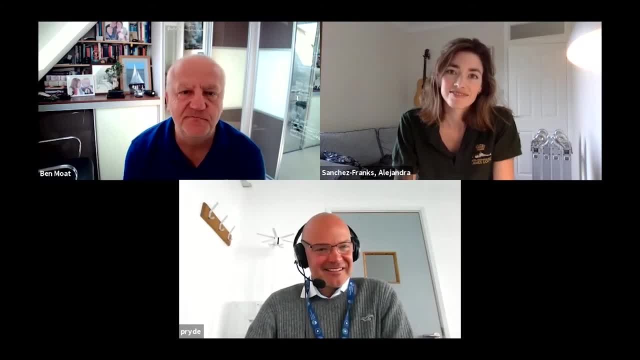 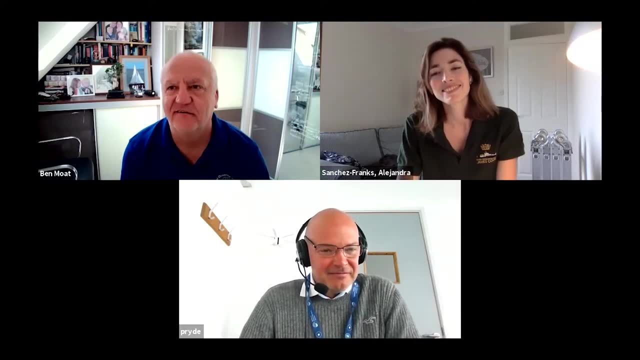 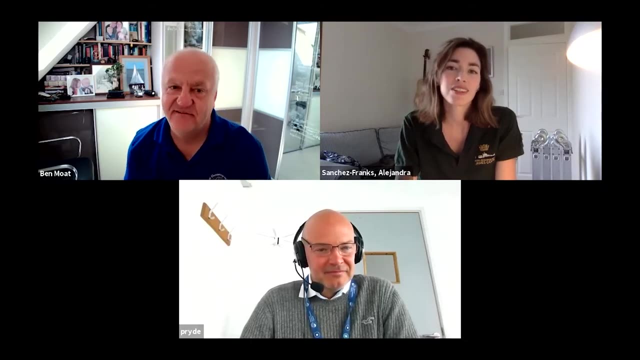 mainly in the North Atlantic. Okay, thank you, Ali. same question to you: what's your favorite ocean and why? I think it has to be the Indian Ocean, which is pretty special for me because it formed a key part in the beginning of my career when I said started to study monsoon dynamics, which 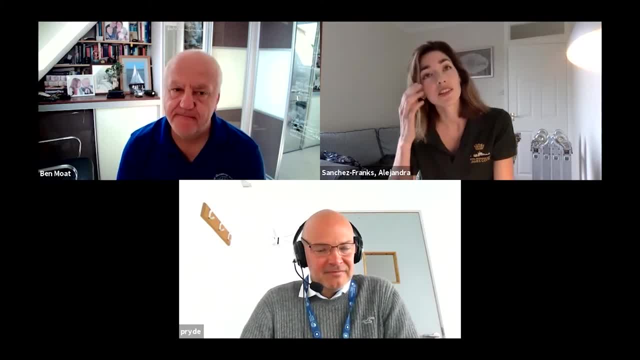 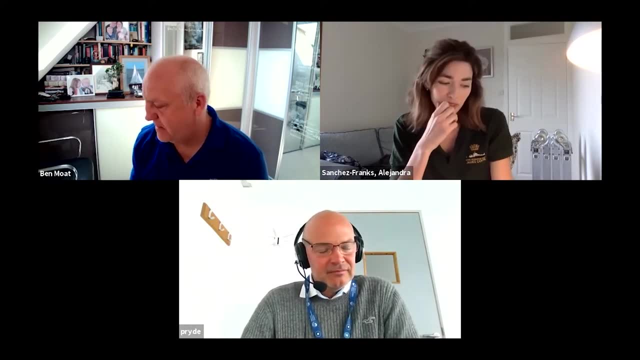 basically affect about a third of the world's population. in the countries that rim the Indian Ocean- And for me, aside from I've so I've done expeditions there which were pretty special and I've mostly focused on tropical oceanography. but but again, you do. 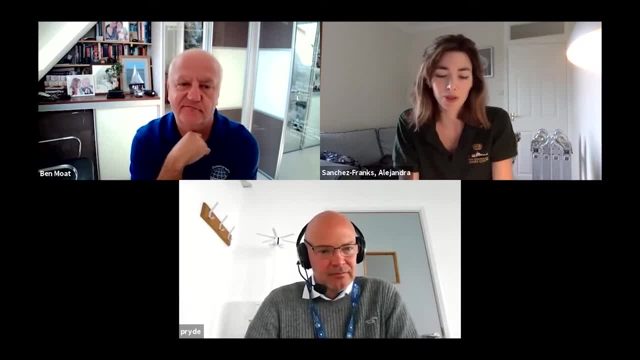 you do see some pretty, you can see some pretty incredible wildlife on tropical oceanography. I remember seeing for the first time a superpod of dolphins which is basically just thousands and thousands and thousands of dolphins, you know, just around the ship in the open ocean. 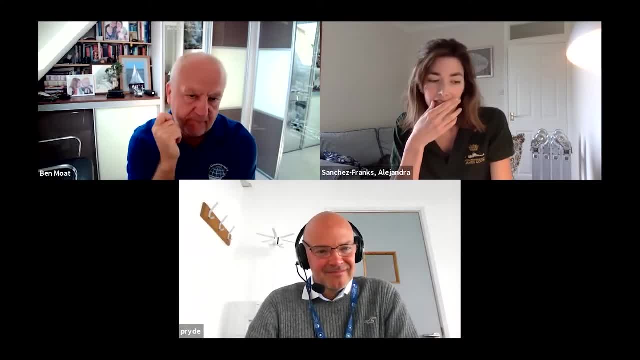 And for me one of, aside from that, one of the key reasons for loving the Indian Ocean is that some of the scientific questions there I find particularly interesting. For example, the Indian Ocean is absorbing excess anthropogenic heat faster than any other ocean in the climate system and it accounts for about a quarter of that global ocean heat uptake. 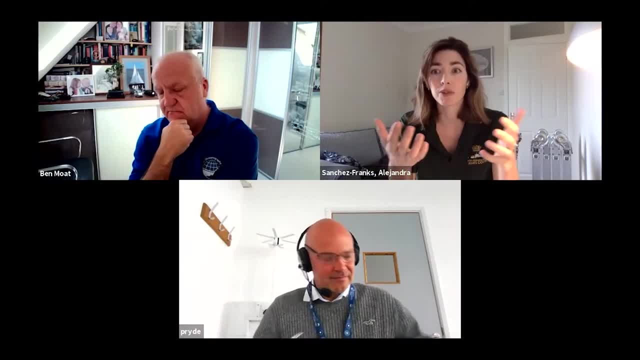 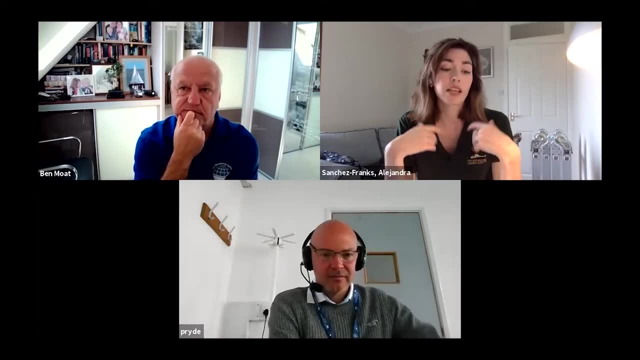 And so now, with the combination of all the new technology that we have, especially available through the NOC, and these questions that are arriving from the global oceans, taking up all that excess anthropogenic heat, makes it a really exciting time to start looking at these things and 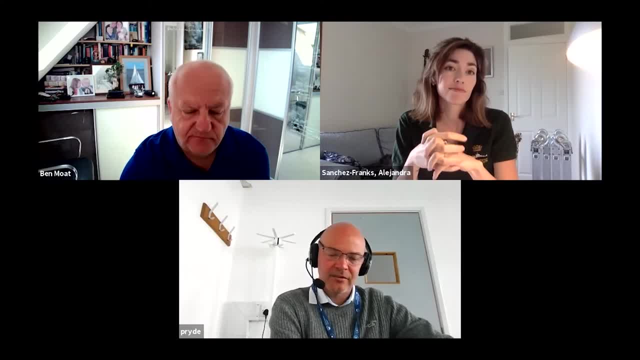 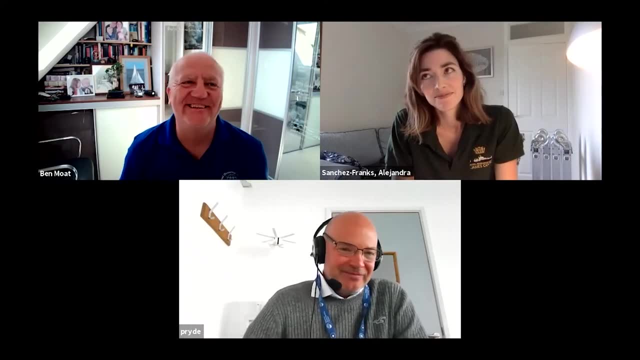 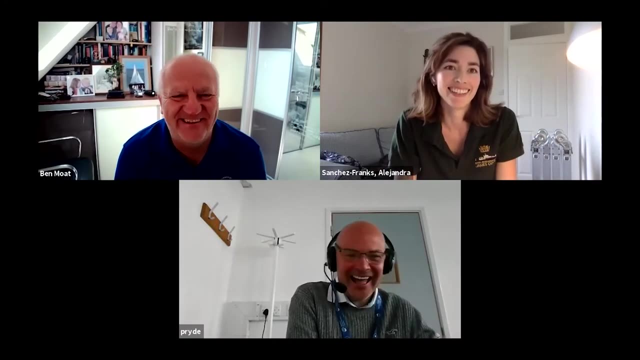 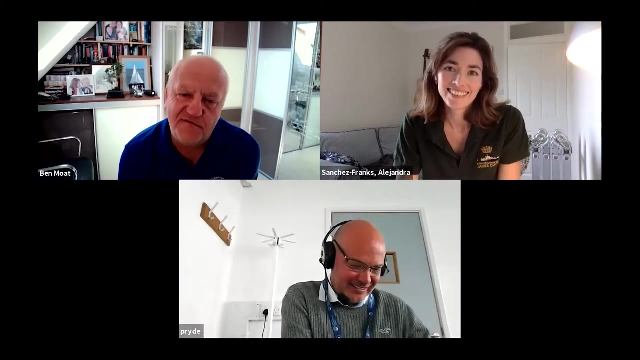 just to be an oceanographer in general, Fascinating. thank you, Ben. how many expeditions have you been on? I don't think I actually know anymore. Ben's an old salt. Perhaps in years is better. So I think I'm around two and a half to three years of my life. 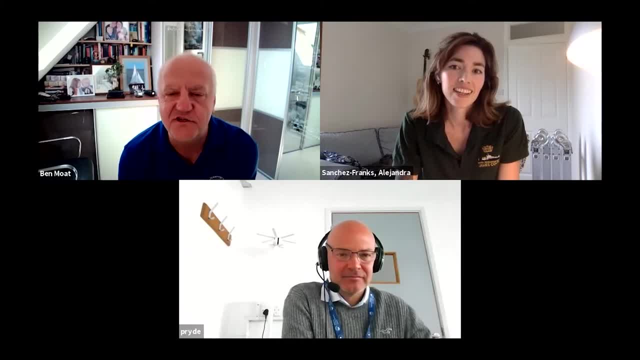 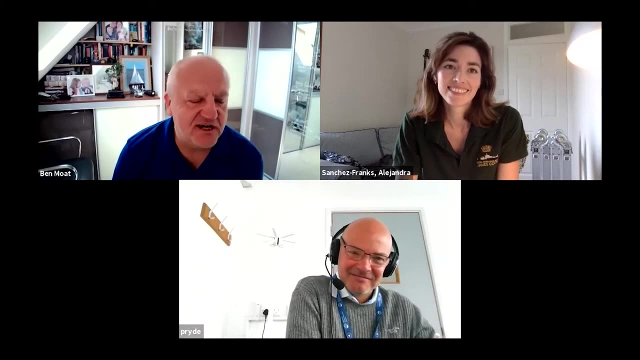 has been spent on that, on our on research ships, I think Maybe closer to three now, but it's yeah, quite a long time, And your favorite would be the one to the Southern Ocean. That was yeah, that was that was good. actually, That was my first trip. 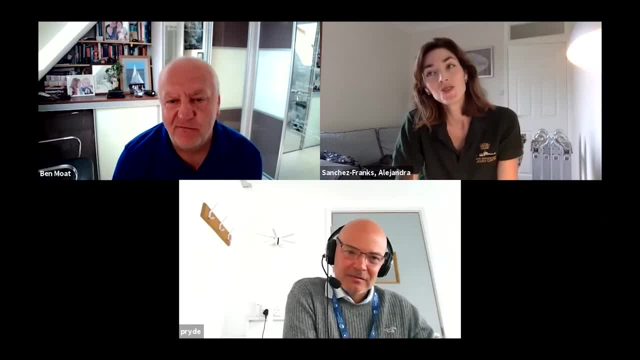 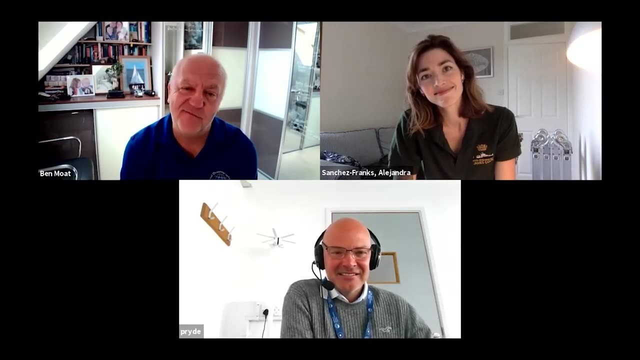 down there. that was back in 1998.. But I do. I have been on trips into the North Atlantic in November, December where we went there for the bad weather and it was really bad But on reflection it was tiring at the time but again that was a great trip, just for the experience. But yeah, I think. 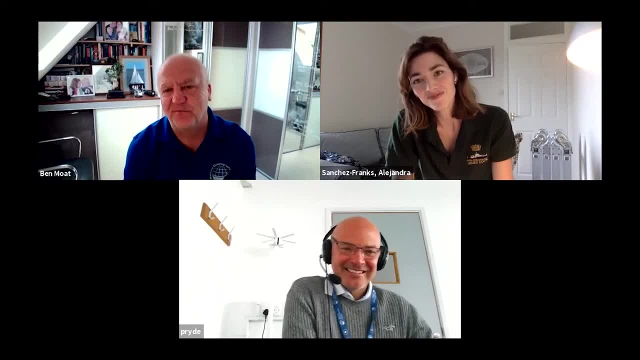 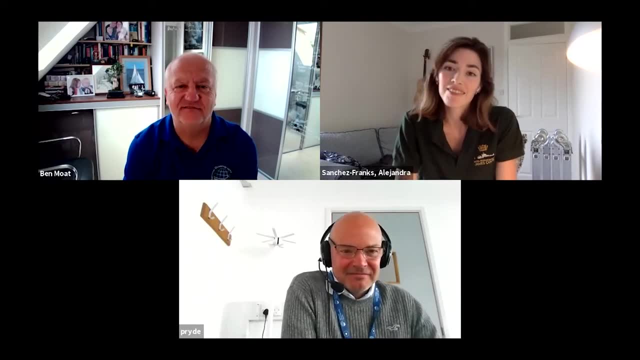 the Southern Ocean? yeah, it's my favorite. I think the Southern Ocean- yeah, it's my favorite. Excellent, Ali, how many expeditions have you been on? I've been on five, One in the Equatorial Pacific going from Tahiti to Hawaii. That was pretty. 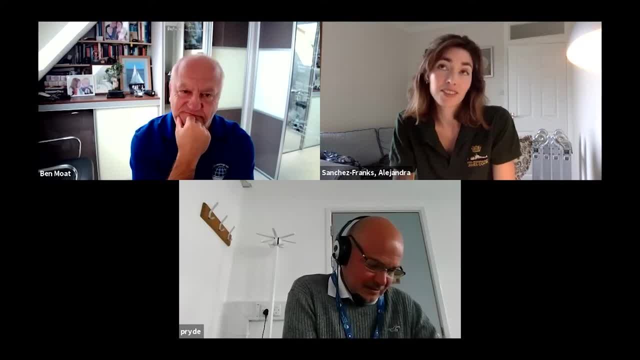 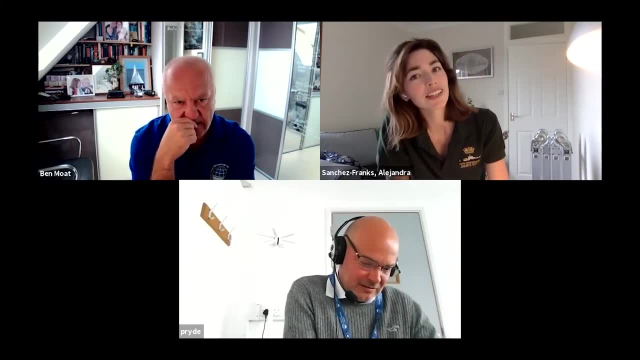 special One in the Northern Indian Ocean, the Bay of Bengal, to look at monsoon dynamics, The South Atlantic, from Brazil to Namibia and Cape Town, and then two in the North Atlantic, And the North Atlantic has been something that I've been really interested in for a long time. I think it's been 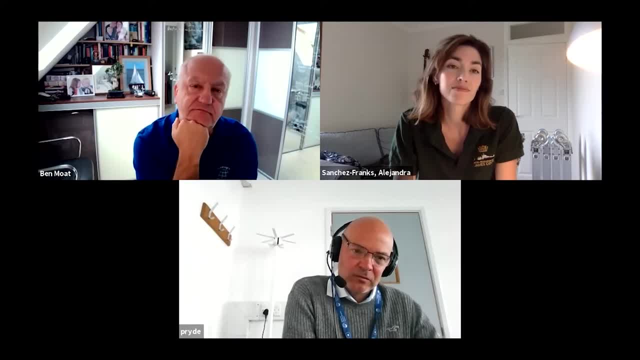 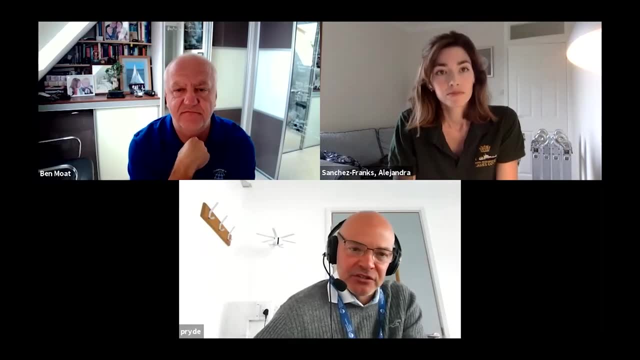 something that I've been really interested in for a long time. I think it's been something that is kind of where we're both focused at the moment. And why are you focused on the North Atlantic? Is that specific to your research or areas of interest? 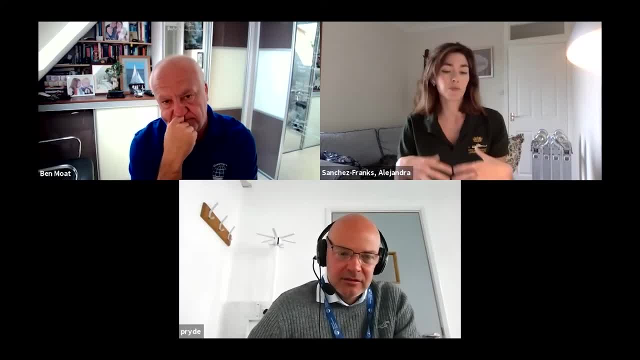 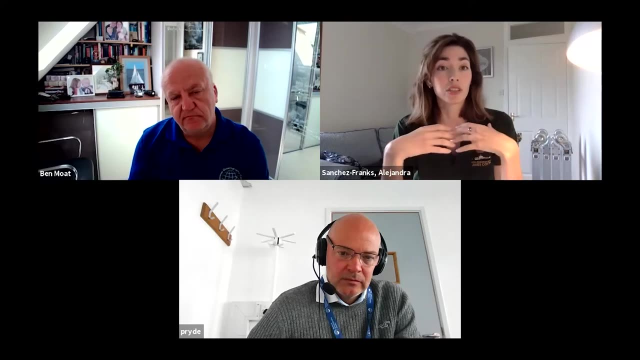 Yes, that's right. So specific to so two things. Both are the areas that we're interested in. We both look at the Atlantic meridian overturning circulation, So basically that has a large focus in the subtropical and subpolar North Atlantic, But also- this is something that the NOC is known- 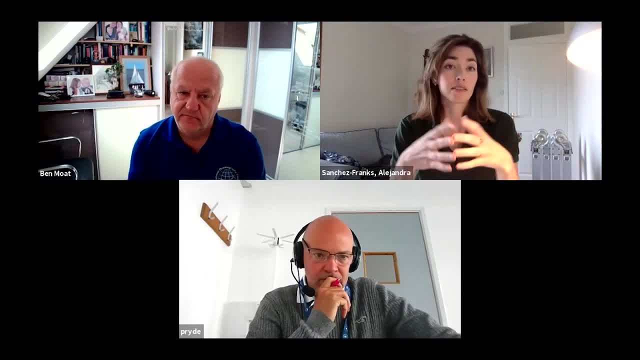 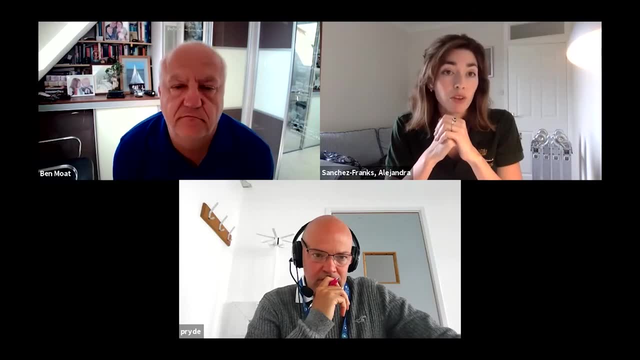 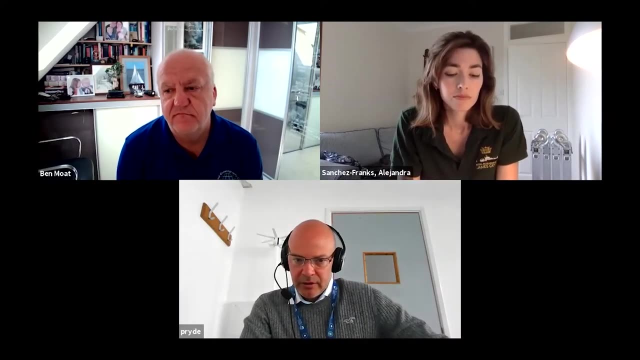 for, Like world experts in the AMOC, and this type of science question is something that we have in our group, So it's a really good place to focus on those questions. Great, So, moving on to a few other questions coming in now, Ben, starting with you, If you could. 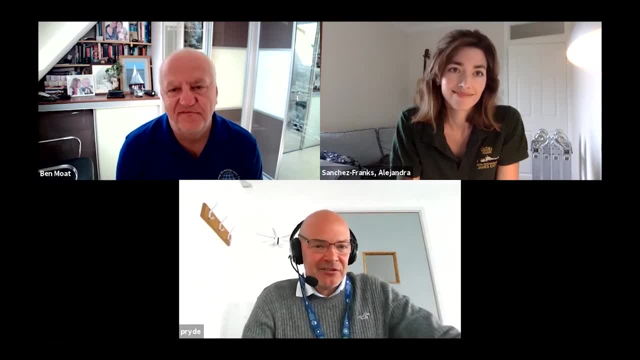 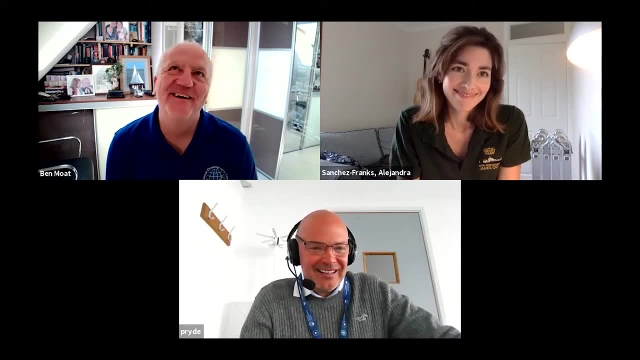 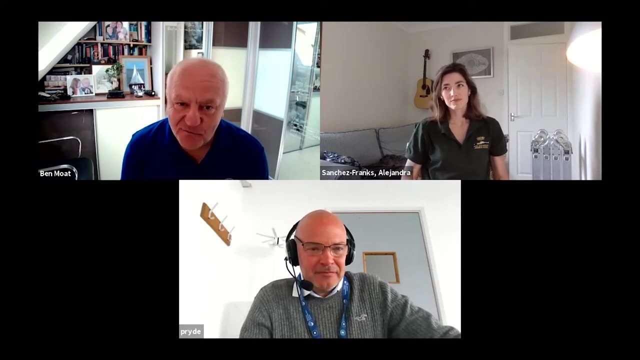 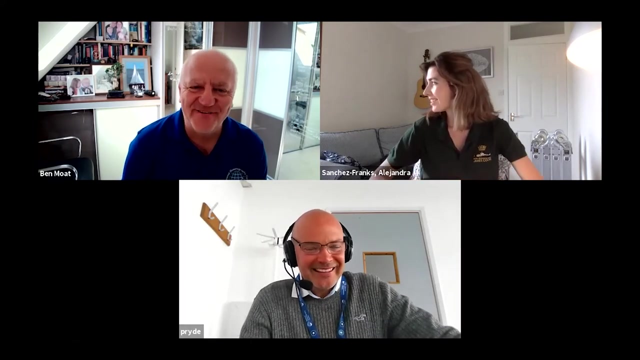 give a 15 year old yourself advice on becoming an oceanographer. what would that one be? Wow, To be an oceanographer. I would say in general, take the opportunities you have that are offered to you, Take them and don't be afraid. You know, go ahead and take those. 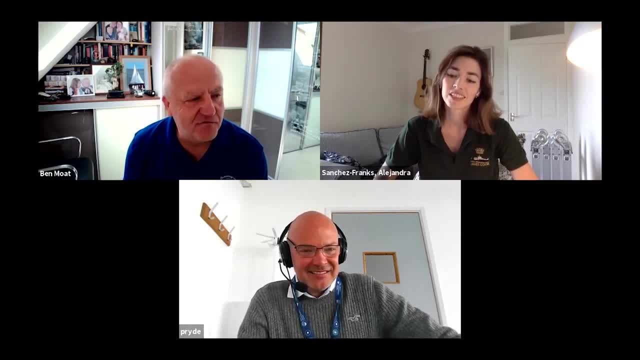 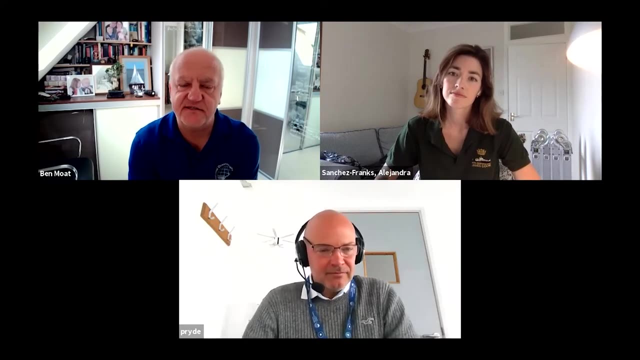 opportunities and go for it. But to be an oceanographer- I think in our talk we highlighted the different disciplines within oceanography- So just pursue what you're good at. You know, if you're good at mathematics, if you're good at biology and you have a passion for the seas, then yeah, pursue what you're good at and what. 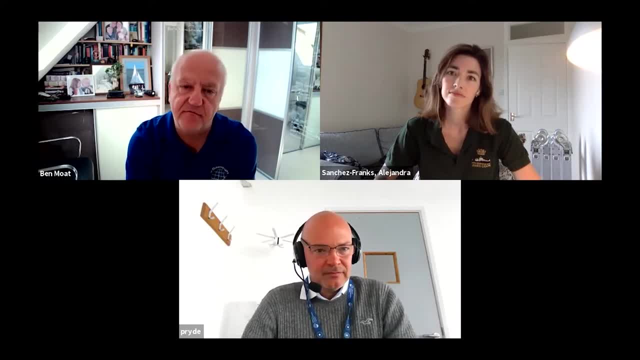 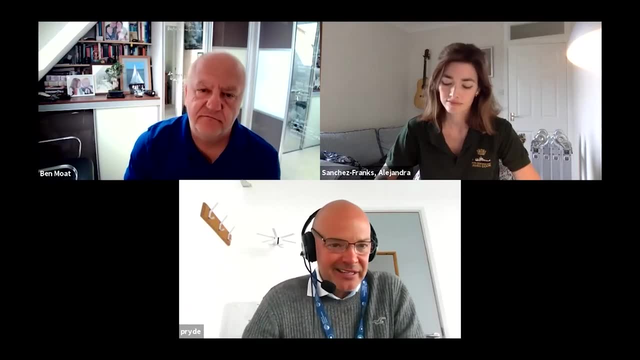 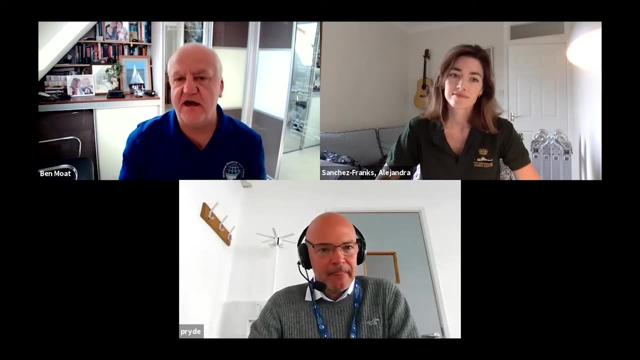 you're interested in And then focus from there, from, say, your first degree within intuitionography. So your core seemed to be mathematics and then the career path seemed to open up from there. is that correct? Yeah, yeah, So I just I was good at maths, so I just focused more on maths and 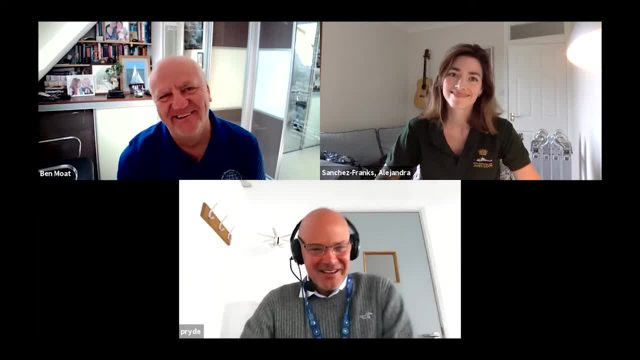 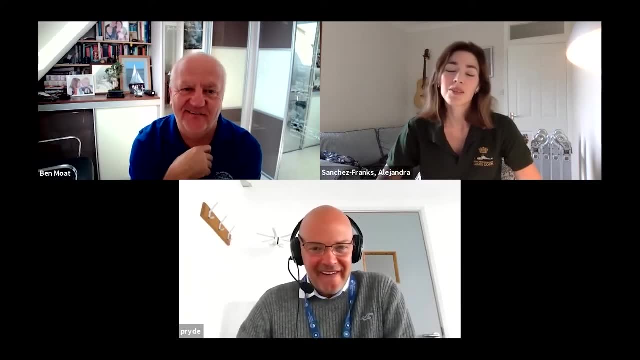 I ended up here, Marvellous Ali. same question: What advice would you give a 15 year old yourself? I would tell myself to get into field work as soon as possible. Just start looking for opportunities for field work, because I didn't get into field work until a lot later. So basically, 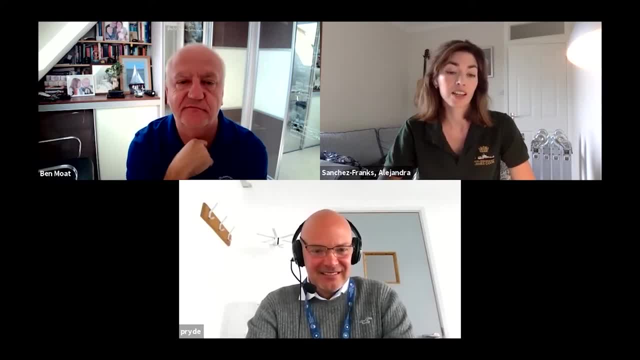 I was ending my PhD and starting a postdoc and you know it's. it's field work is so amazing and there's so many opportunities to join and there's different types of science that you can do, or technical or technical roles if you're more interested in that. 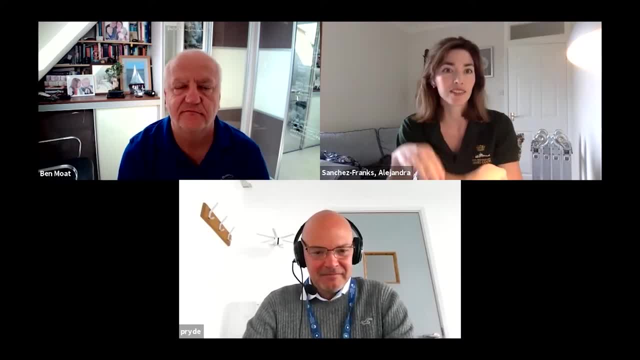 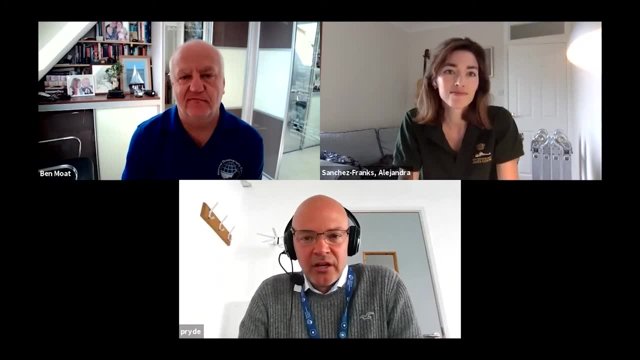 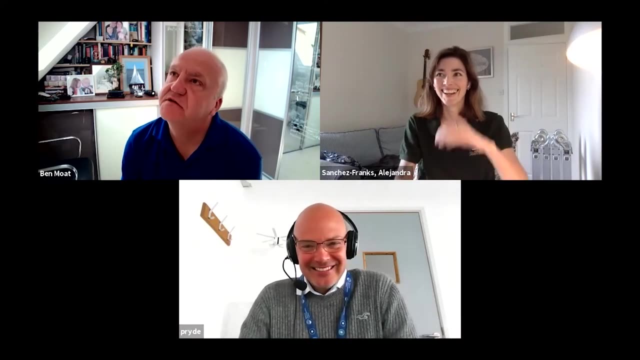 And so, yeah, that would be my advice, just like: look for the opportunities and take them as soon as you can. Fantastic, and had you both had working at NOC on your radar as a place where you wanted to end up, Ben. So, when I first started the, actually the institute, the- 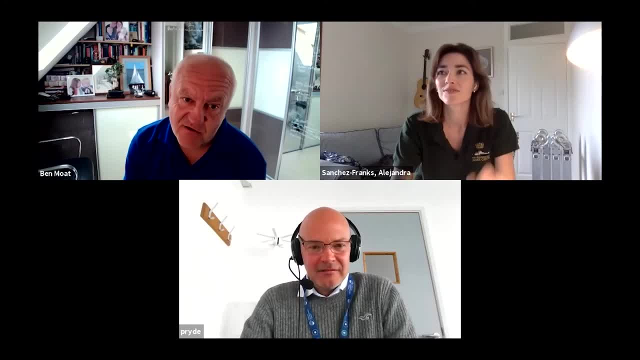 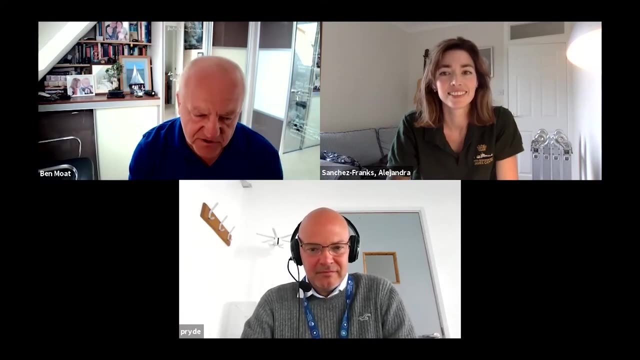 oceanographic science was in the middle of Surrey, so that was the sort of UK focus. then we had different institutes around the country and they came together to focus in about well, pre-95, 93 probably, it was just you know- the focus was to build this oceanography centre in Southampton. 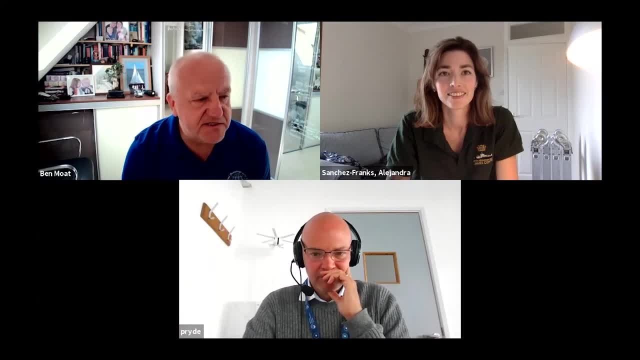 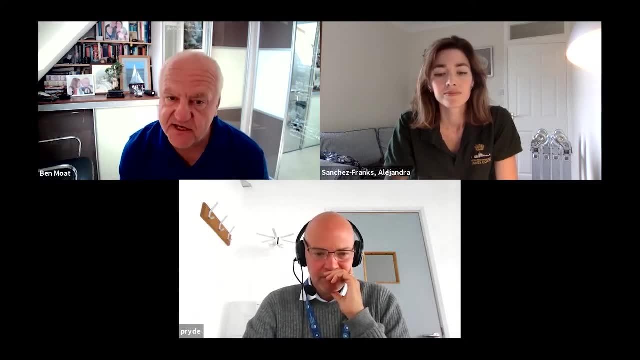 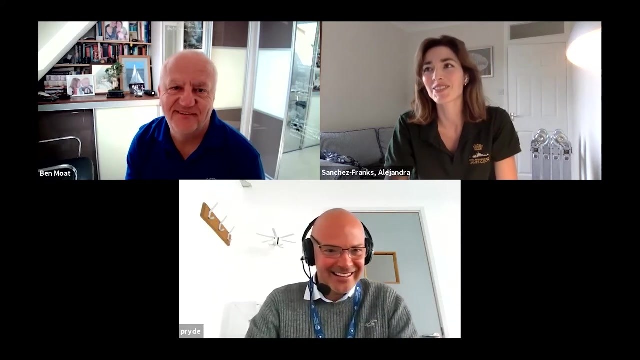 So, yeah, I would say it was more focused towards this, the institute oceanographic sciences and the, the SSC as it was then, yeah, rather than I would say a university. I had my eyes on on that specifically. yes, yeah, Right, same question, Ali. I'm so glad Ben's going first so I can think about. 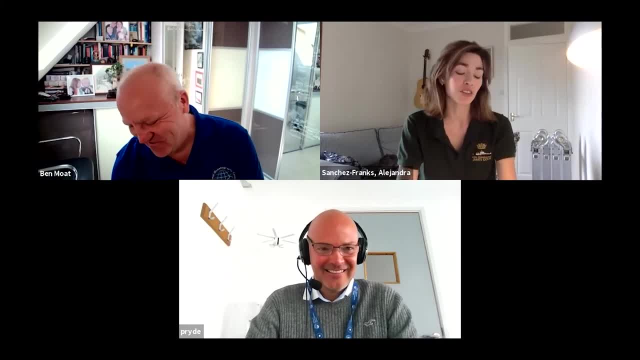 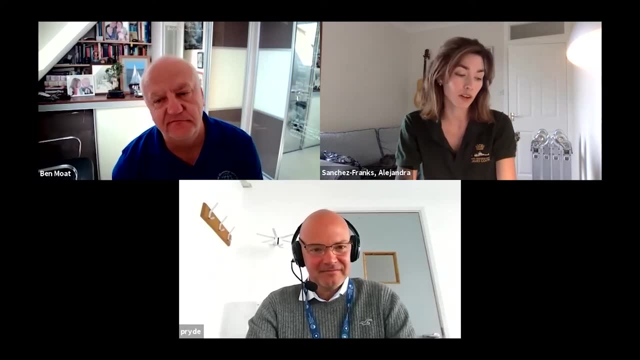 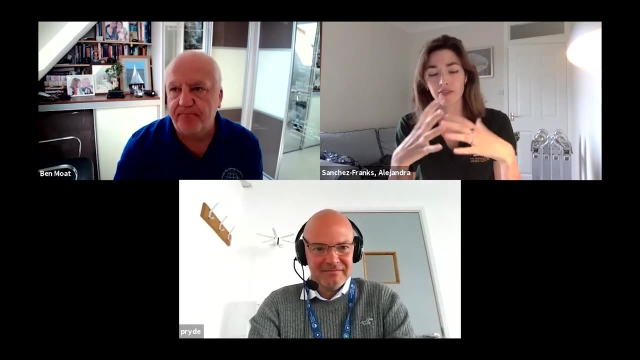 these things? No. so the truth is no, because I wasn't really aware of this type of career path when I was at university. but once I'd started my- once I started looking into oceanography as a profession or, you know, getting into oceanography PhDs- you know life after that. 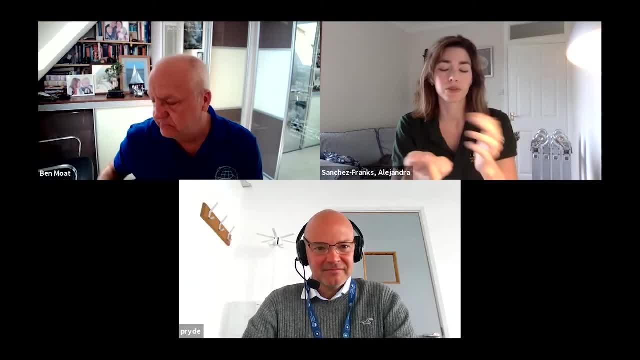 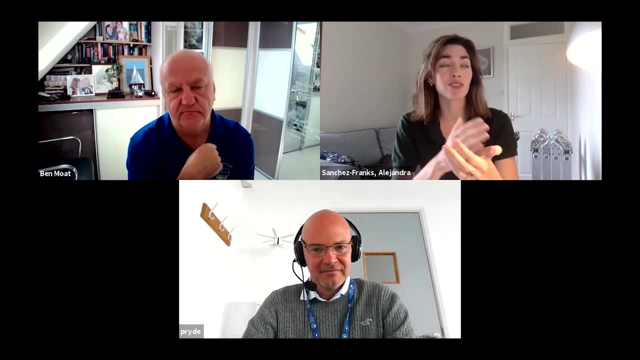 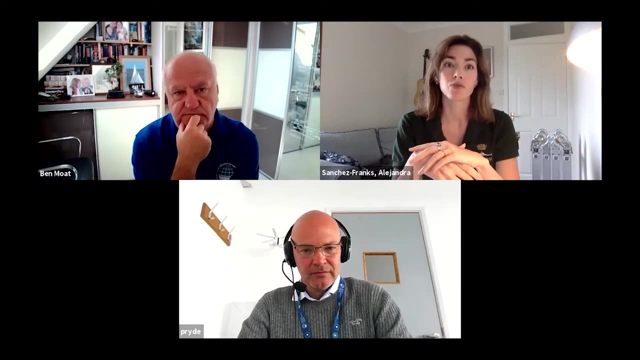 it was definitely. it definitely came on my radar along with other top oceanographic institutes in the world like HUI or Scripps and- and critically, one of not. it was on my radar not only because it was one of the top institutes, but because it had a lot of resources for doing a lot of different. 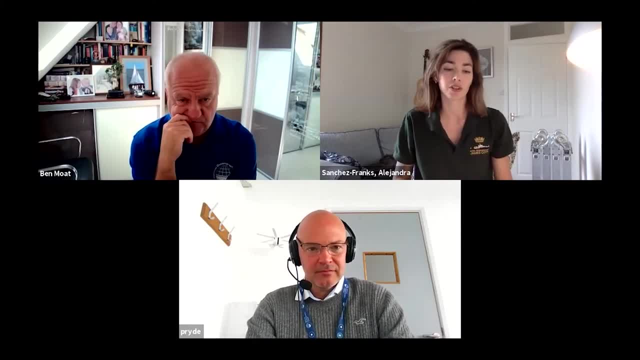 types of science. So I think most people go through things early on in their career or their life where they're not really quite sure what they want to do for the rest of it. So you want to be at a place where you have a lot of options to maybe. 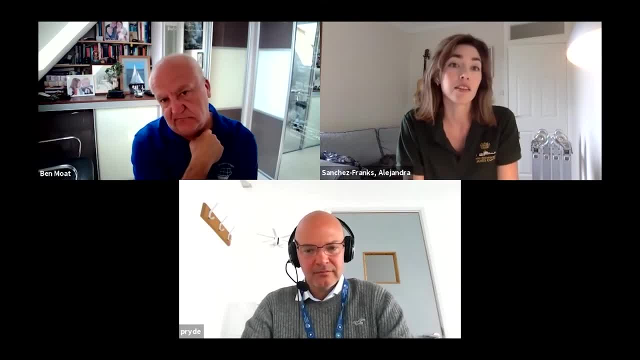 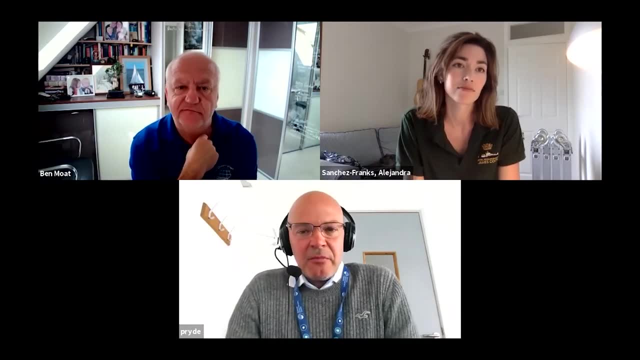 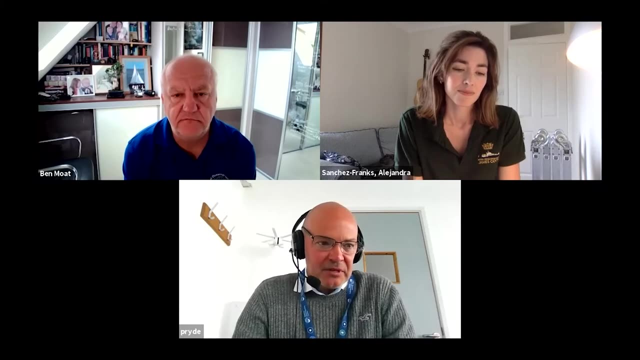 change your mind or try different things or get different advice. and the NOC- you know the NOC had all those elements. Okay, well, you're both very passionate about the career paths you've taken and the work that you want to take. I think, if you could maybe just just summarize what 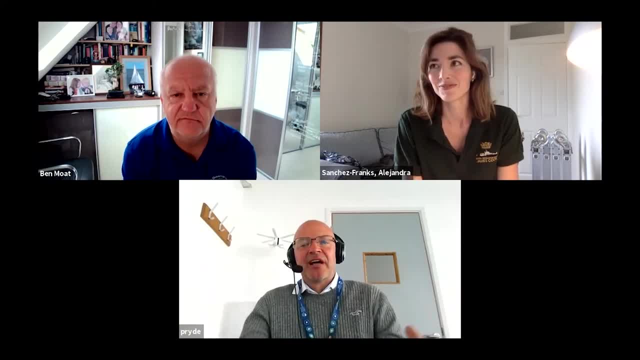 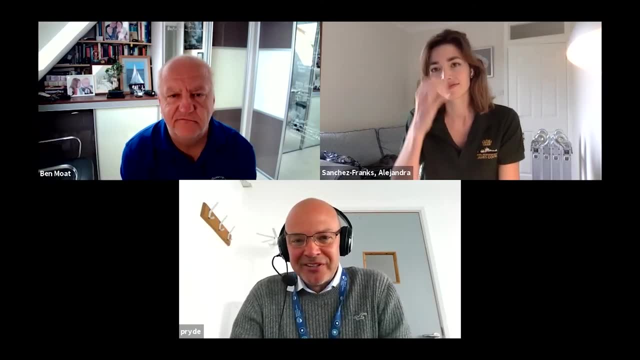 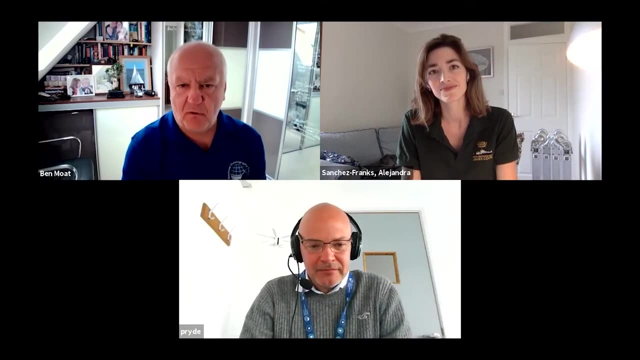 makes life special for you, whether it's a you know different day, or the fact that you're finding other or new findings, new research. you know just what makes it special for you. Well, within oceanography, you know, I think I've never had a single job that always not remained. 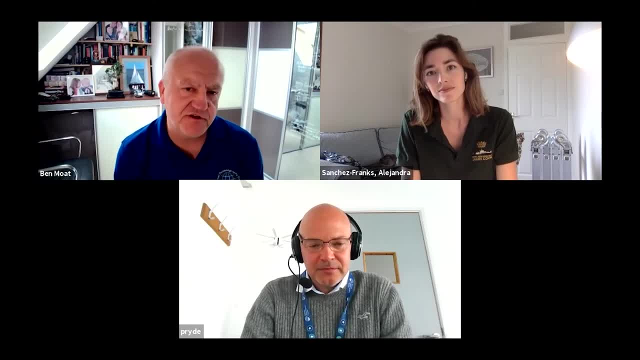 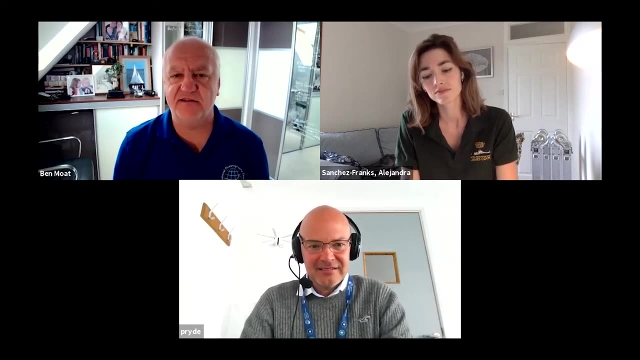 the same. within oceanography, I've always worked on different projects in different oceans with different goals, so it's like you never get tired of this. You're right, you're always discovering, just finding out new things, and these things we find, they have. they have meaning and impact. 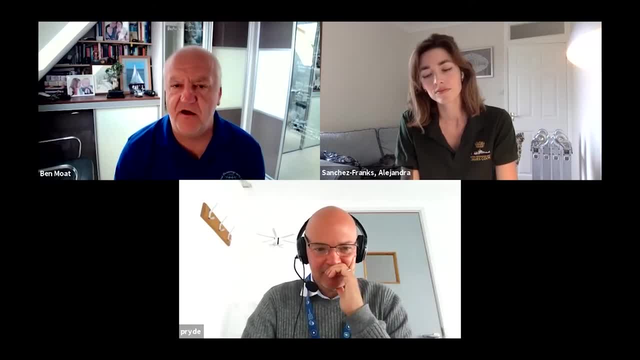 because you know we need a healthy ocean to support the fisheries. You know, as we said in the talk, 50% of the air we breathe is from the ocean, so we need a healthy ocean. So that's our focus. our aim is to work out how the climate is affecting our oceans and what's the impact on us. 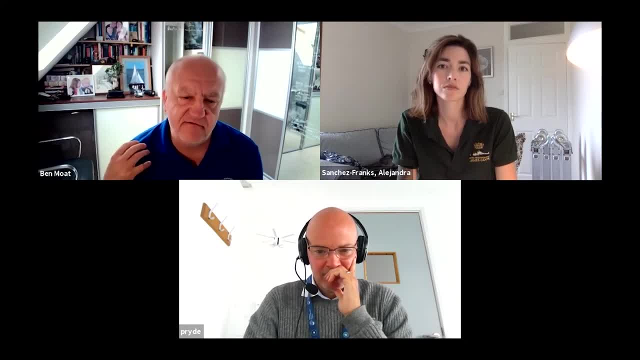 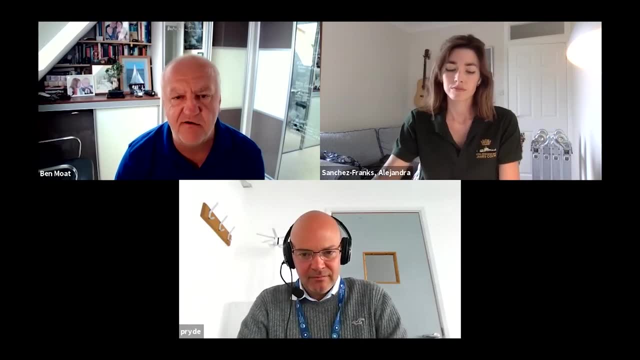 As I say, it's a job in oceanography, it's. it's. whatever projects you're working on, it's always different. you know you take the same skills between different projects, but you're always learning something new. I don't think, as scientists, we ever really stop stop thinking or trying to work. 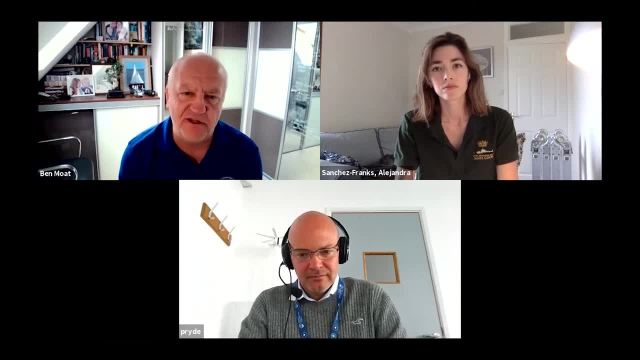 things out, ever since you know you can, walking along the beach and suddenly come up with a solution for something you know and you know, so it is as a career is very, very interesting and and very, very rewarding. So not your average nine to five, No, no. and we've talked about research ships as well. you know the research ships, as Ali said, runs. 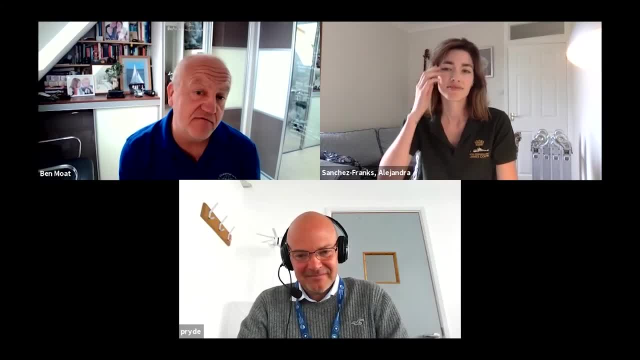 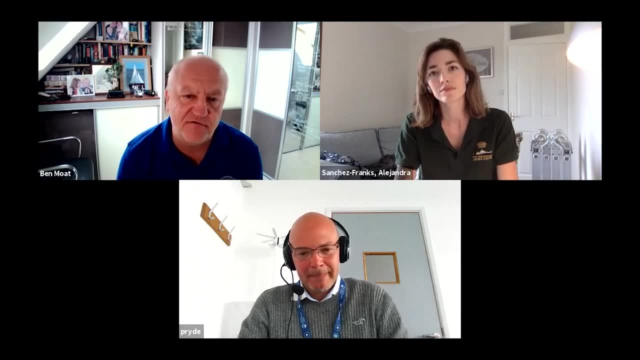 24 hours a day. You know you'll be working an eight or even a 12-hour shift, but everything the science is is just carrying on and you bounce our ideas off, our ideas off each other and your feet. you know ideas for papers, for journal papers, or even projects or questions. we don't know the. 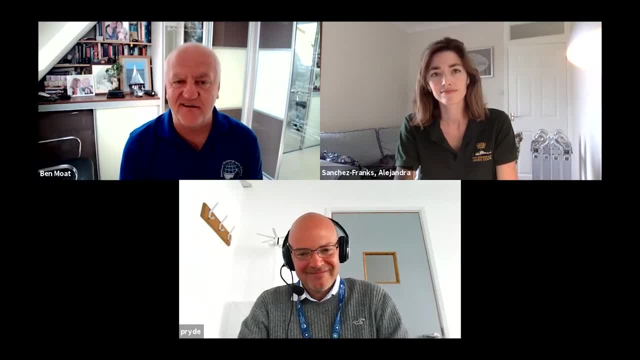 answers to. You can be there at four in the morning having a cup of tea, just looking at the ocean, and suddenly come up with something like: why don't people thought about that? and yeah, take it from there so that'll inspire you to to get some funding in and look at that research. 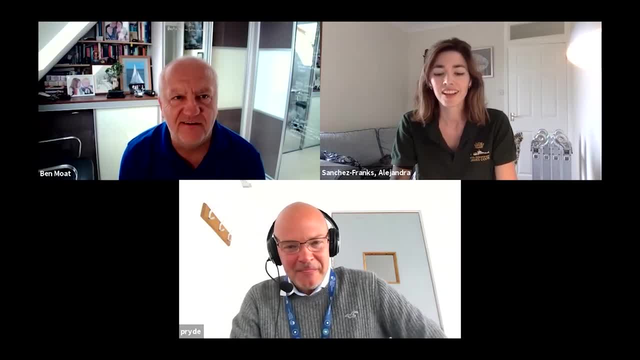 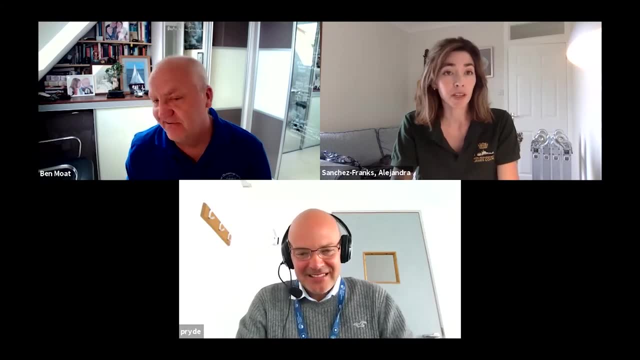 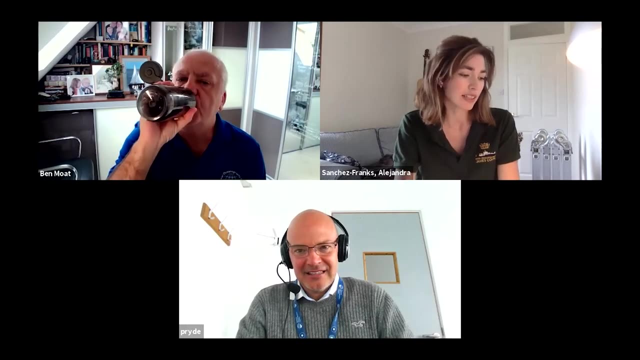 Marvellous. yeah, Ali, same question: what do you love about your job? Ben put it really well: the field work, the real world implications of the things that we do, which you know are very tangible and they're things that we can see. I would add to what Ben said that I don't think a lot of people realize just how new a field 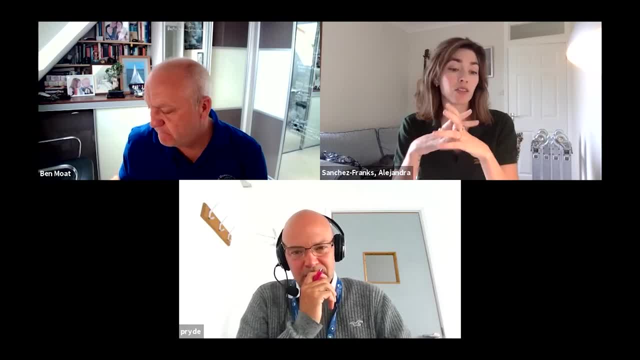 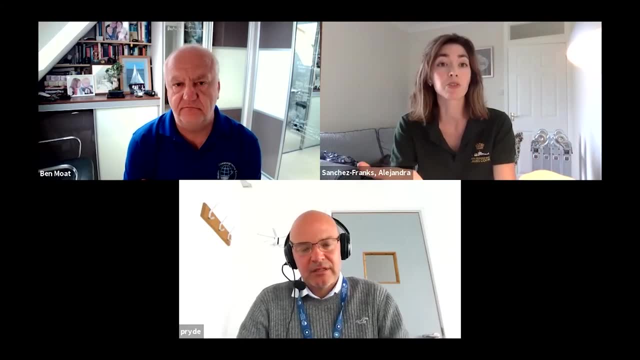 oceanography is uh, and what that means is, you know it hasn't been that long. you know, compared to other science, like atmospheric sciences, that we've had direct mesh, direct observations of the ocean and the data that we're using to now answer really big questions. 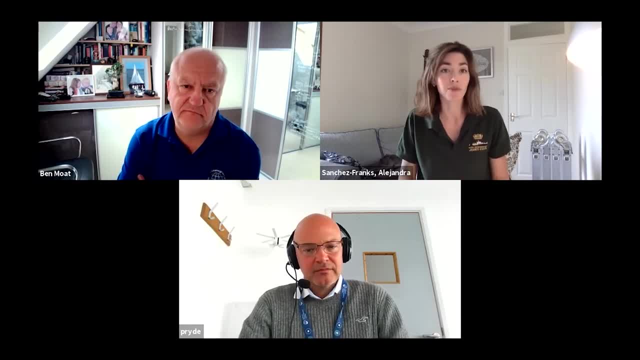 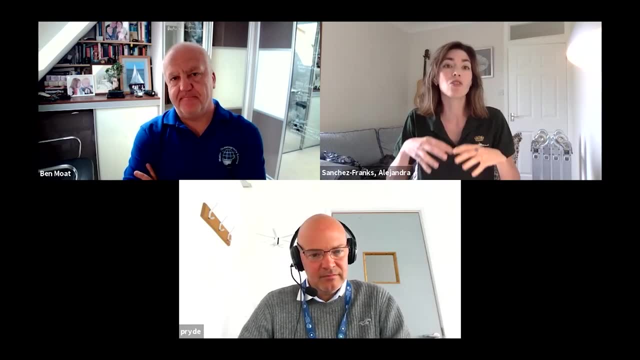 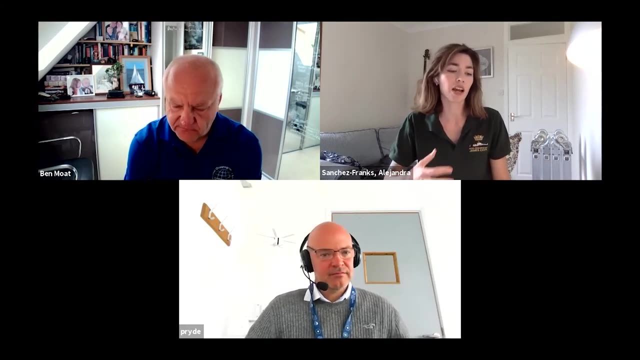 So what this means it's, it's a really exciting time to be a pioneer in answering, you know, these oceans, these questions on ocean circulation, because no one's done it before. you know it's only been, you know it's only really been the last few decades, the last 50, 100 years where you know. 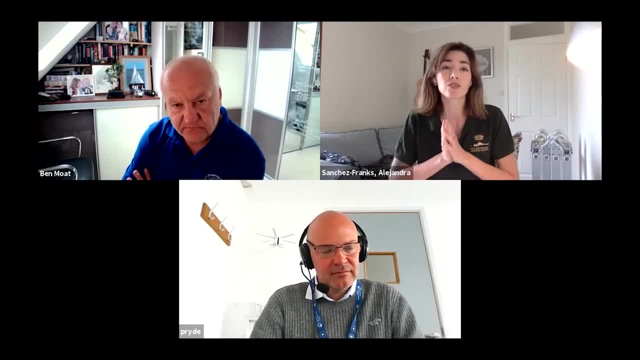 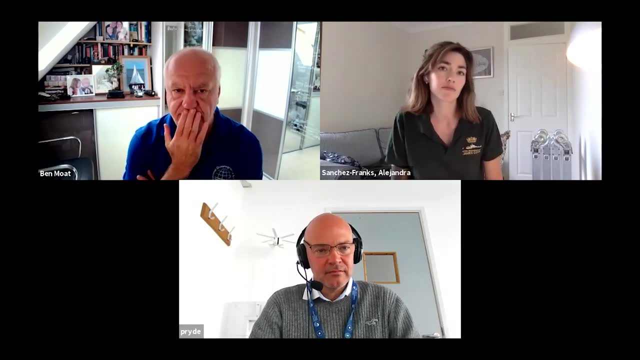 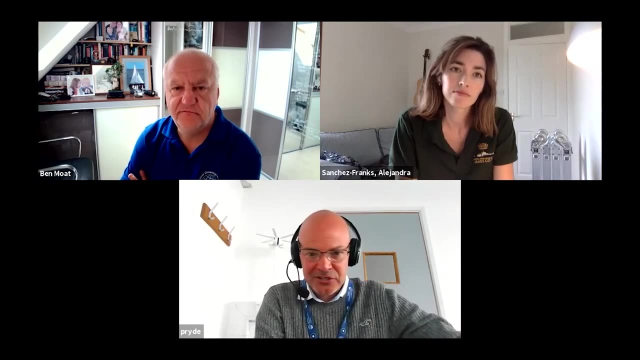 this. this is really grown as a field, and so this means that there's just so many things that are unexplored and so many questions to ask and and and be in a good position to answer. Yeah, yeah, absolutely. I think we'll try for one one last question, um. so question to you, Ben. 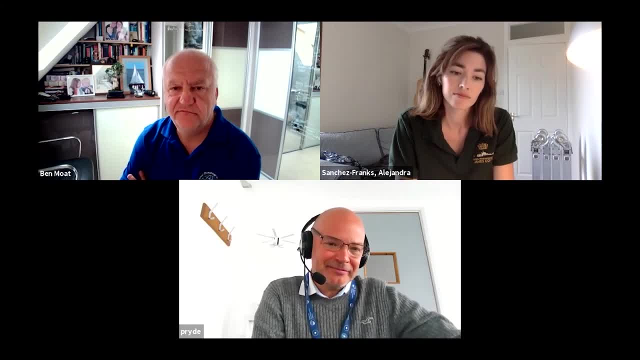 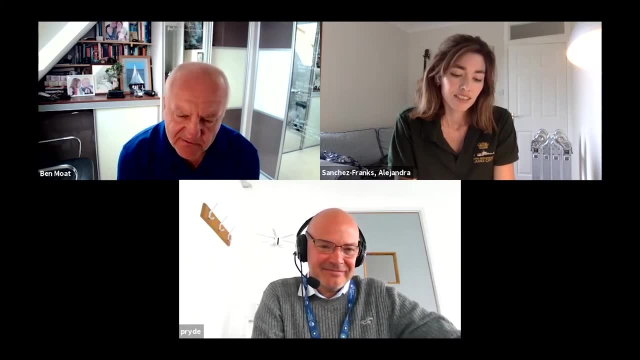 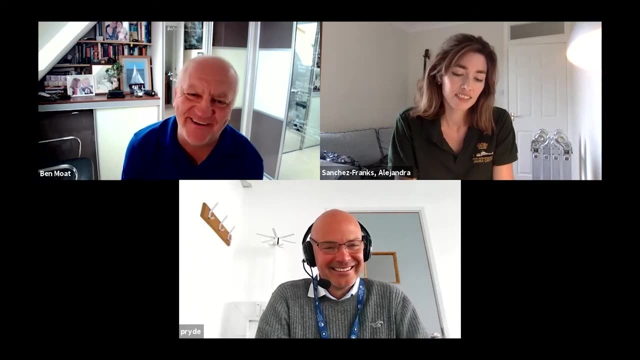 Um, who's been the most important person on your journey? Wow, I would say. thinking back to school, I would say there was a maths teacher who really sort of pulled me up- by my bootstrings, if you like- and got me, and got me on this, on the path to oh made. 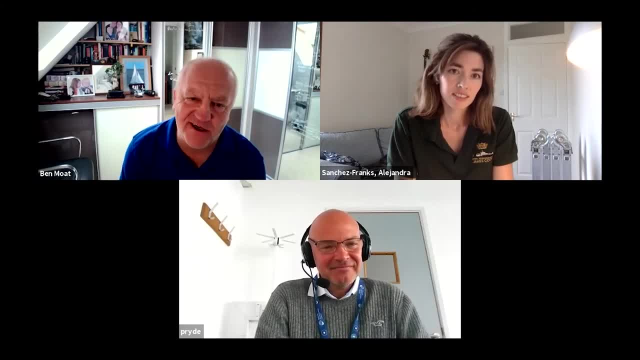 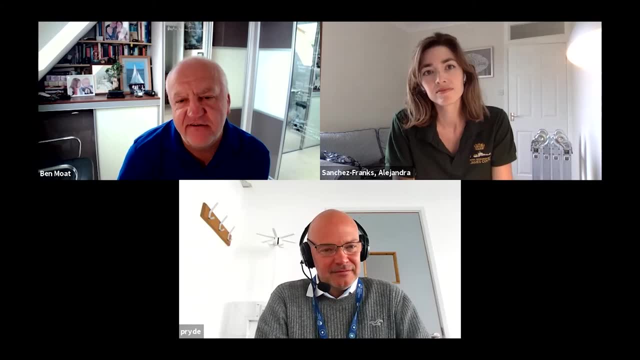 I think, made the best of my passion and really focused me and got me working on maths problems and but it but in but in oceanography. I remember looking at these, these scientists who led these long cruises, these basin scale cruises, you know, across the islands in the pacific and in the atlantic and you even now I go back and I used 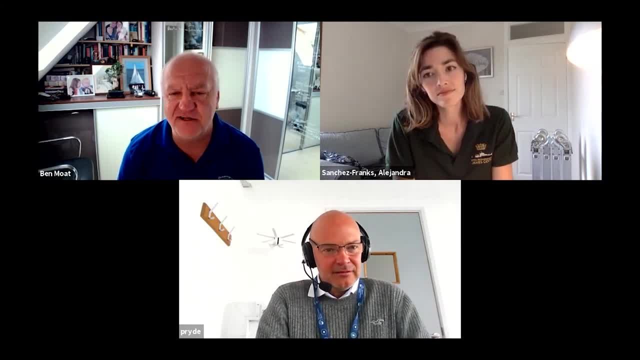 to talk to them and they this: they were just to me. it was fabulous and fascinating. you know they would. we didn't have the Argo program in those days so we didn't know the structure of the ocean or how the structure of the ocean changed. so every time they went out they found new things, new, new.